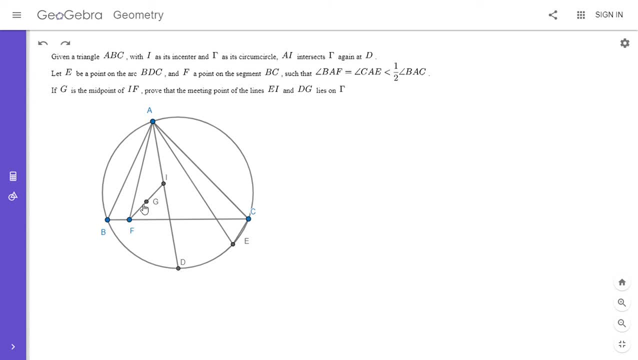 those two lines. but if we extend EI and we extend BG, we want to show that that intersection point lies on the circumcircle. So I really enjoy this problem because I feel like it's a great example of how to use spiral similarities- or at least my solution involves spiral similarities pretty. 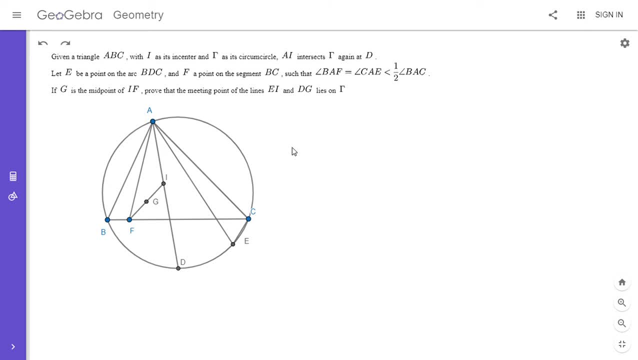 heavily, And I feel like it's a great example of how to use spiral similarities- or at least my solution involves spiral similarities pretty heavily And I feel like it's a great example of how. I've never done a video yet on spiral similarities, but I'm going to have to soon because I keep 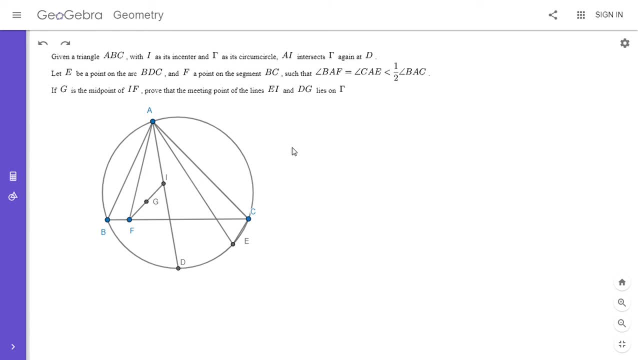 using them over and over in my solutions. All right, so how do we get started here? So whenever I have the in-center and the midpoint of the arc, opposite angle A, for example by the in-center-ex-center lemma, there's a circle centered. 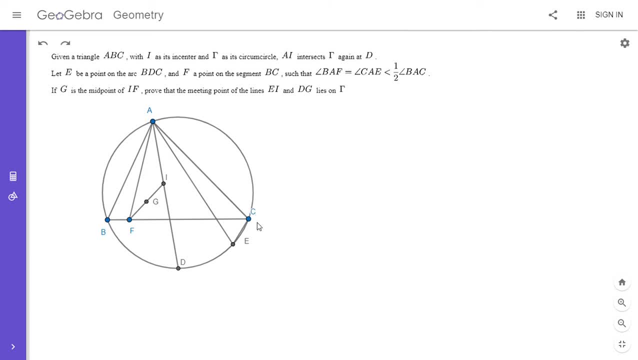 at D, passing through B, I and C. And not only that, it also passes through the X-center opposite A. So I'm going to write this out. I mentioned this in one of my recent videos. I've never proven it, but it's a fairly well-known fact. So D is the midpoint of arc BC and by this lemma, 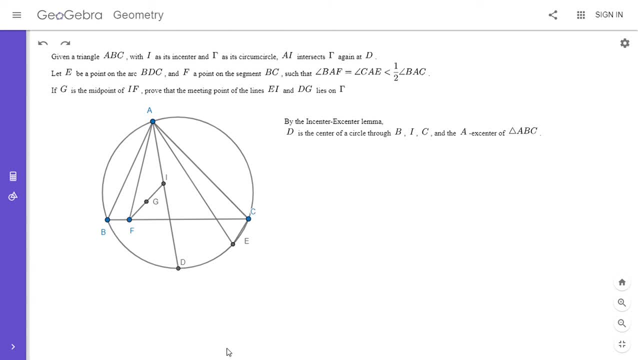 it's the center of a circle through B, I, C and the AX-center. So I'm drawing that circle centered at D. So H is the X-center opposite A, So it lies on the angle bisector from A, And I don't even really use the fact that it's the X-center in my proof, but that happens to. 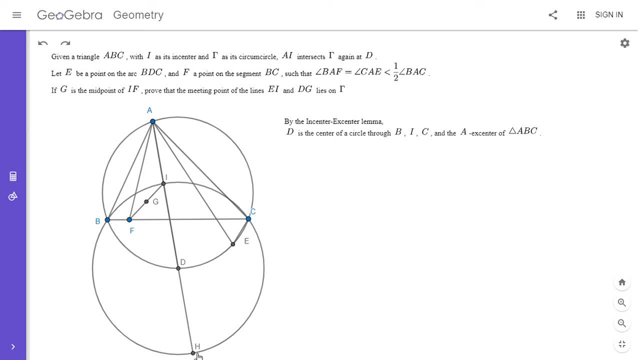 be part of the lemma. So, basically, I'm letting H be the intersection of A, D, with this circumcircle through B, I and C, And so IH is the diameter. All right, So where do we go from here? Well, so we want to try to use the fact that G is 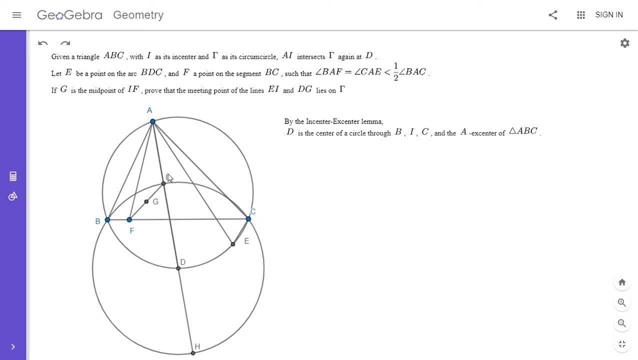 the midpoint of IF, And my idea was: we know that IB is equal to DH, since D is the center of the circle and those are both radii. So that means that DG is parallel to FH. So that is how I'm going to use that fact. So, since IG is equal to GF and IB is, 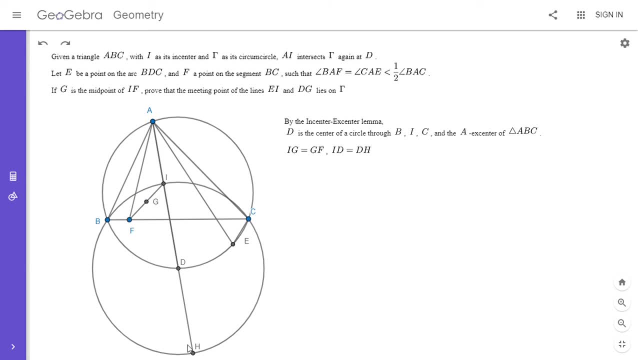 equal to DH. that means DG is parallel to FH. Okay, All right, So I'm going to draw on those two segments. And now, how do we ultimately show that the intersection of EI and DG lies on gamma? Well, if you look carefully, that's the same as saying that angle ADG is equal to angle AEI. 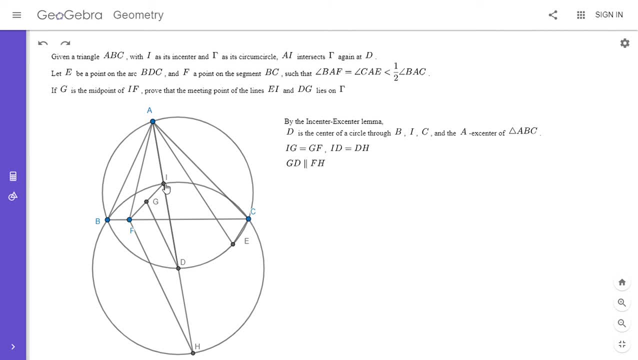 Because if that were true, that those two angles were equal, then if you took the intersection of them, if you let them intersect at a point K, that would mean that AEDK would have to be cyclic, And so K would have to lie on the. 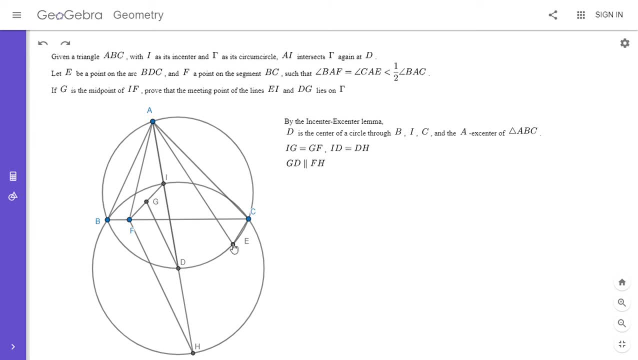 circumcircle. Okay, So really we want to show that angle AEI is equal to angle ADG, But from the parallelism angle ADG is equal to angle AHF. So we want to show: angle AEI is equal to angle AHF. And so we want to show that angle AEI is equal to angle AHF. And so we want to show: 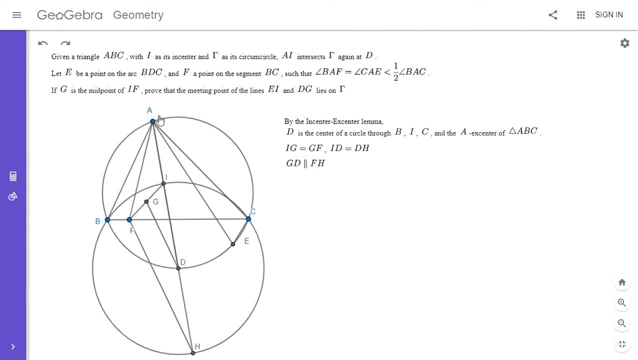 angle AEI is equal to angle HF, And so we want to show that angle AEI is similar to angle AHF. Okay, And now we want to show signal A That we did not input, We did not include at the end. 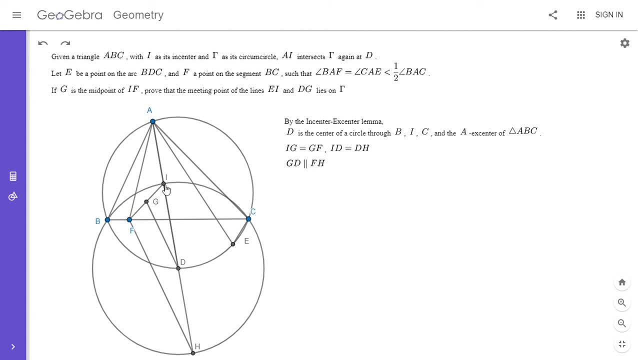 to show that it's going something like that. So we want to show that it's going to look like that And that it's not hard to see. that's the same as showing that those two triangles are similar. So we want to show that. triangle AEI. 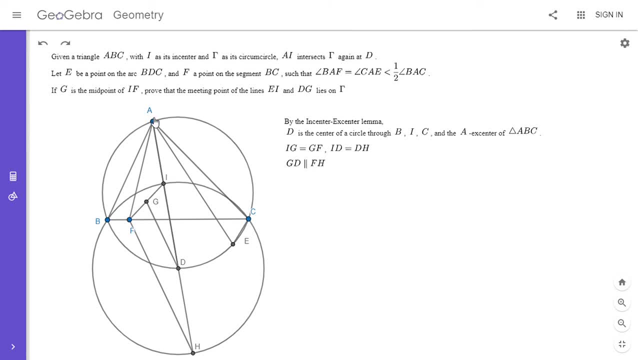 that's equivalently the same as showing that triangle AIF is similar to triangle AEH using properties of spiral similarities. So that's how I'm going to go about it. I want to show that triangle AIF is similar to AEH. Okay, and I'm going to start by doing something very similar to what I did in video number 63 on my channel. 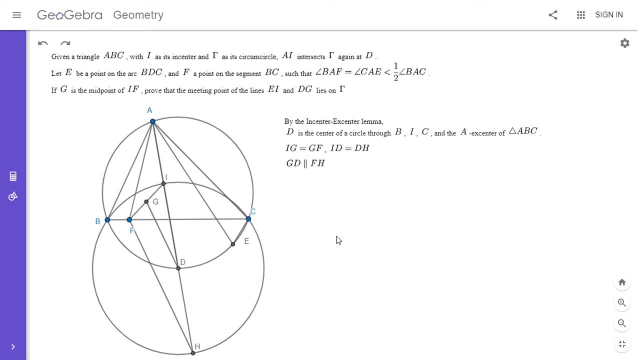 So if you haven't seen that video, I'd recommend checking it out. But basically, the first thing I'm going to note is a pair of similar triangles, triangle ABF and triangle AEC. So those are both similar triangles And that's not hard to see. so I'm going to show that through an angle chase. 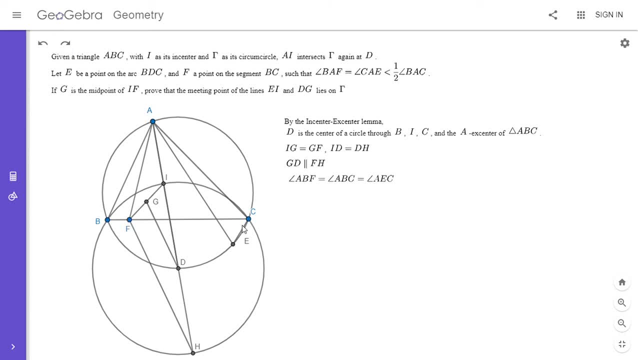 So we have: angle ABF is equal to angle ABC is equal to angle AEC. So in triangle ABF and AEC, we know that that pair of angles is equal. And another pair of angles is also equal from the problem statement Because we're given in the problem that angle BAF is equal to angle CAE. 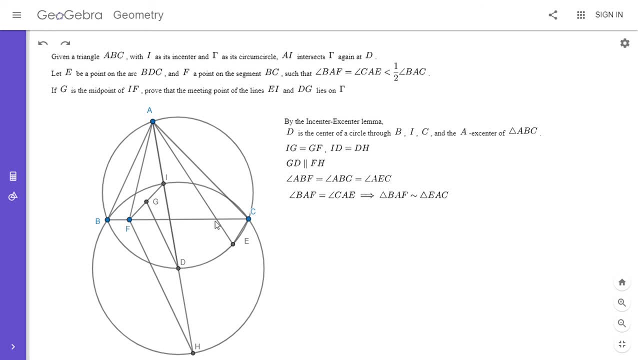 So that means that triangle BAF has to be similar to triangle EAC And if that's true, that means there's a spiral similarity that takes triangle BAF to triangle EAC, Because they're both joined at point A and have the same orientation. 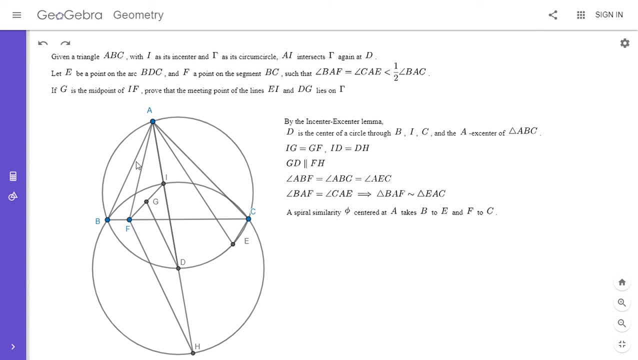 So a spiral, similarity, phi- that's centered at A, takes triangle BAF to triangle EAC. So, in other words, it takes point B to point E and it takes point F to point C. So then, what I'm going to try to do. 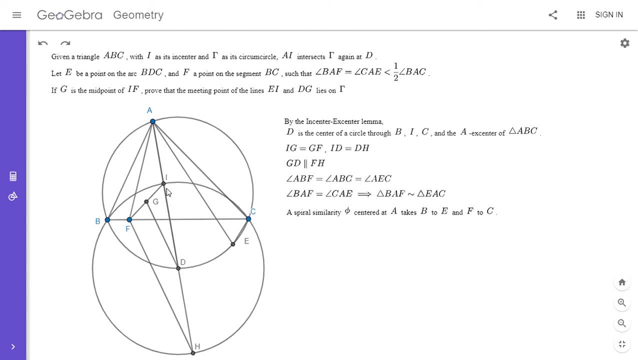 Is. I'm going to try to see where does this spiral similarity take point I? So I'm going to let it take point I to a point J, Just like I did in video 63 on my channel. Okay, So let the spiral similarity phi take point I to point J. 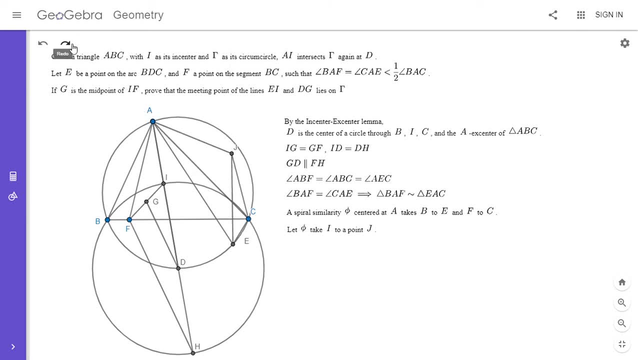 So I'm going to construct point J. Okay, All right. So that means that the whole quadrilateral ABFI is similar to the whole quadrilateral AE ECJ through the spiral similarity. All right, So how do we make progress from here? 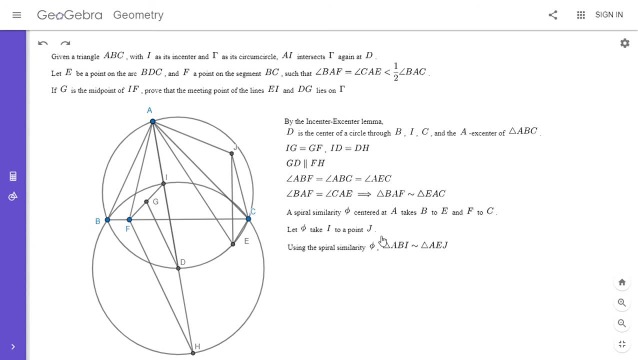 So, using the spiral similarity, like I said, the whole quadrilaterals are similar And so we know that triangle ABI is similar to triangle AEJ. That's another fact that we can derive from the spiral similarity, because those are corresponding triangles and those two similar quadrilaterals. all right, but I claim that triangle ABI is. 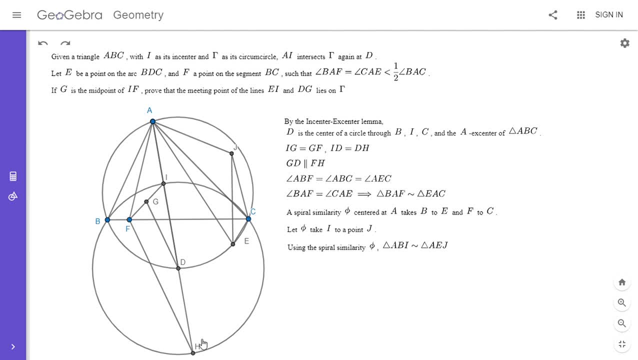 actually similar to triangle AHC and that's also not a very hard angle chase, so I'm going to do that right here. so we have angle ABI is equal to angle IBC, which is equal because BI is an angle bisector and IBC is equal to angle IHC. 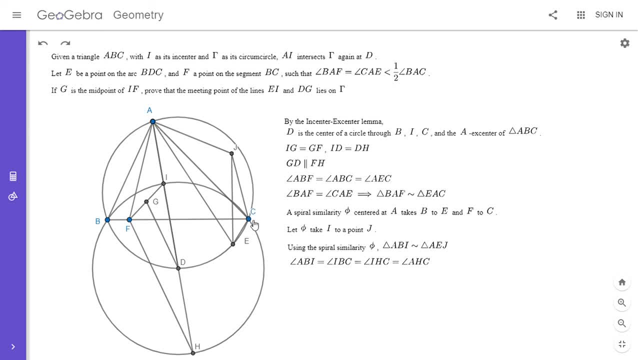 and obviously that's equal to angle AHC. so the two triangles, ABI and AHC, they both share this angle and it's easy to see they share another angle. so angle BAI is equal to angle AH. this should be. angle BAI is equal to angle. 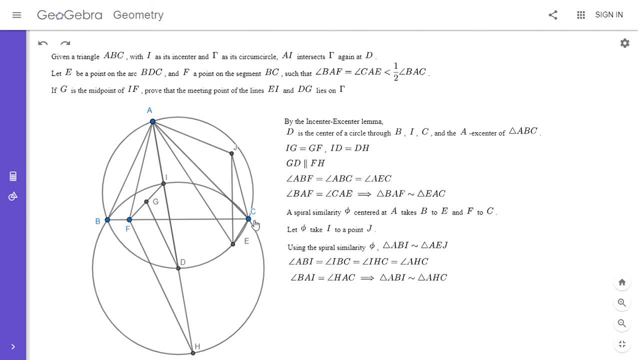 IBC. Oh yeah, that's correct. angle HAC, because AI is an angle bisector, And so triangle ABI is similar to triangle AHC. okay, because two of the angles in it are equal, All right, and so we said previously, though, that ABI is similar to AEJ. 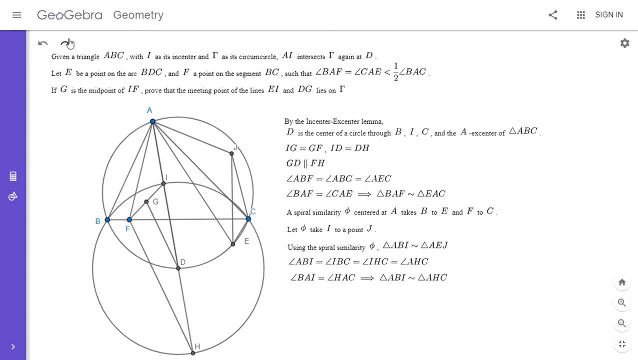 So that means that triangle AHC is similar to AEJ, So I'm going to write that out here. So we have these three similar triangles and now we can use facts about spiral similarities, but on these last two pairs of triangles. So if triangle AHC is similar to triangle AEJ, then that means the spiral similarity takes one to the other. 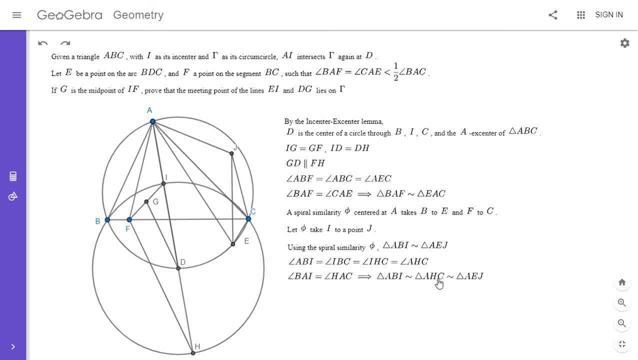 So using properties of spiral similarities, we can sort of interchange the points other than A and we would get that triangle AEH. So triangle AHC is similar to triangle AJC. all right, So lots of uses of spiral similarities here. So I may do a video of this on my channel. but basically you can, since triangle AHC was similar to triangle AEJ. 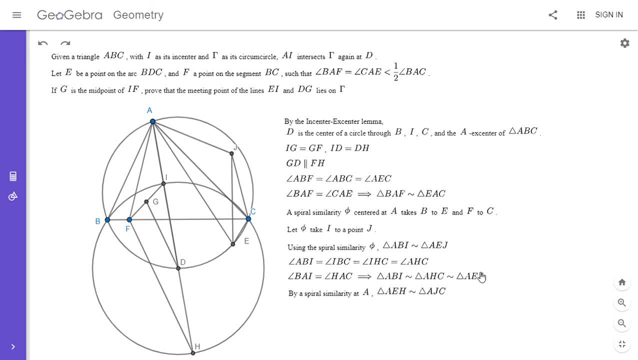 if you swap points E and C here by the properties of spiral similarities, you get another pair of similar triangles. So I will do a video. I'll be back on this fairly soon. All right, so triangle AEH is similar to triangle AJC. 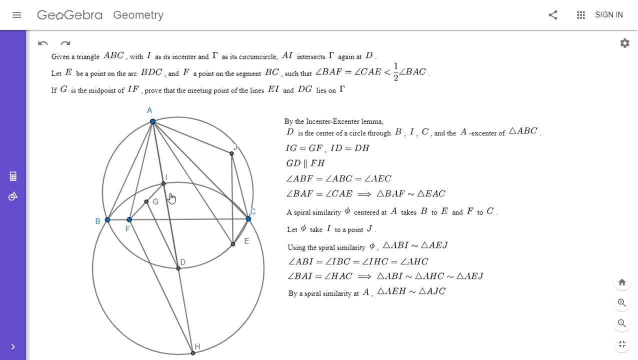 and triangle AJC is similar to triangle AIF because those, like I mentioned, these two quadrilaterals are similar, and so those are AJC and AIF. Those are corresponding triangles in those two similar quadrilaterals. Okay, so we have triangle AEH. 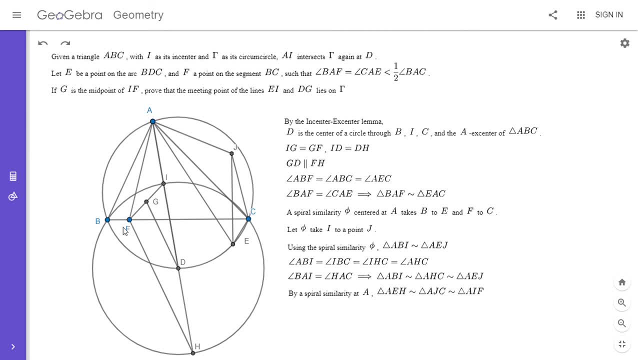 and triangle AEH is similar to triangle AIF, And now we can use a spiral similarity yet again interchange the points, as I mentioned. So, with the triangles AEH and AIF, since those are similar, using properties of spiral similarities. 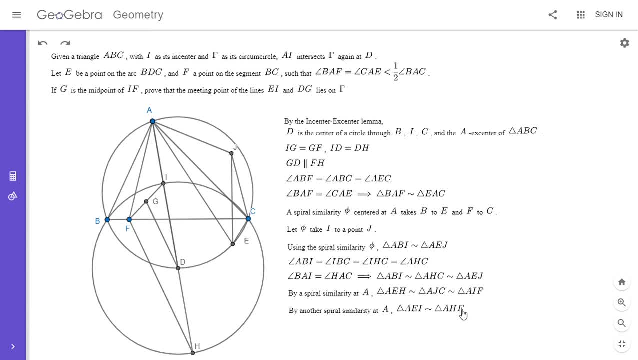 we then have: triangle AEI is similar to triangle AHF. By swapping, by moving I to this triangle and H to that triangle, we get another similarity. And this gets us exactly what we want, because if triangle AEI is similar to triangle AHF, 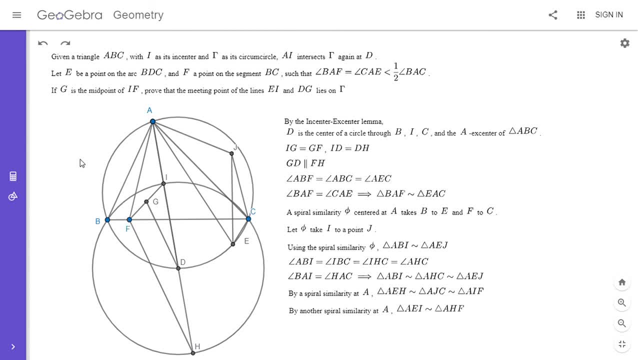 that gives us the two angles that we wanted to be equal, because now we can do an angle chase, which I'm going to show you, So just drawing in another segment. So angle AEI is then equal to angle AHF, since those two triangles are similar. 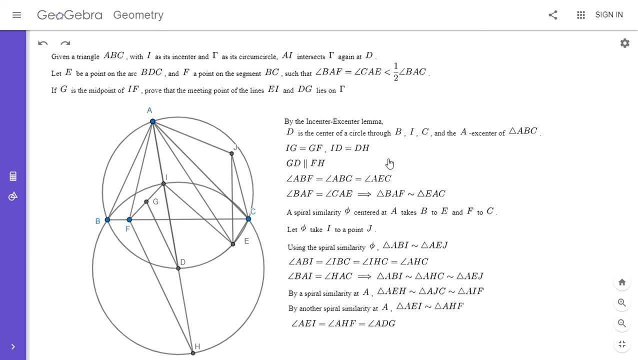 and that's equal to angle ABG, Since GD is parallel to HF. So we have angle AEI is equal to angle ABG And that's enough to show that EI and DG have to intersect at gamma. Because if EI and DG intersected at a point K, 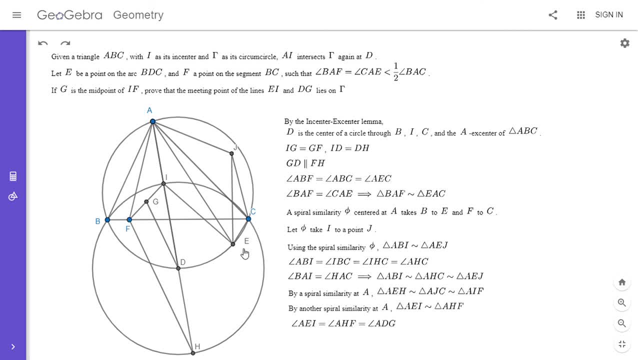 then from this angle equality we'd have: angle AEK is equal to angle ABK And that would mean AEBK is cyclic. So in other words, the intersection of EI and DG has to lie on gamma. So I'm going to call that K. 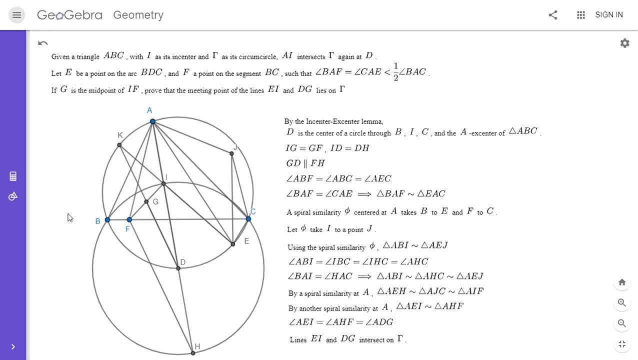 So I thought this problem was a very cool application of spiral similarities. There's another subscriber to my channel, Osman, Now, and he has a YouTube channel of his own where he shows a different solution to this problem, So I'm going to show a link to that.